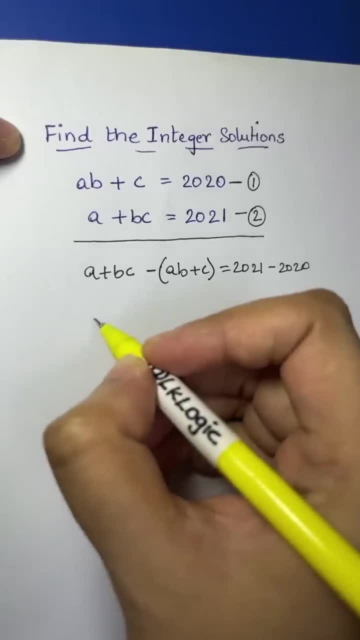 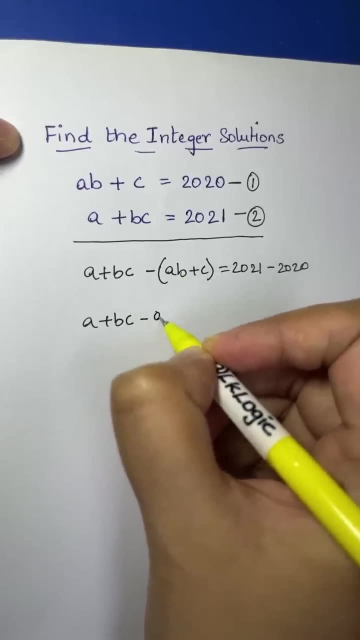 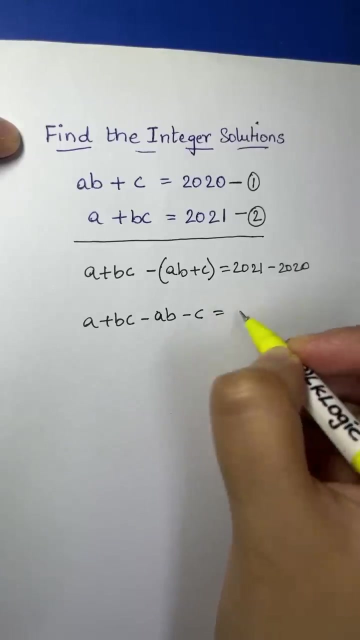 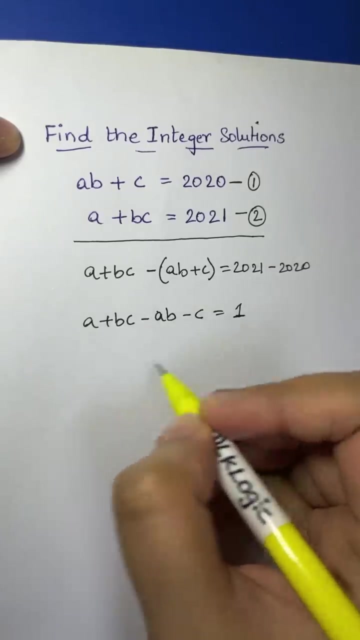 All right now. what do we have? Just open up your parenthesis- a plus b, c minus into plus minus minus a, b minus into plus minus c equals to 2020.. 21 minus 2020 gives you one. All right now. what do we have? Can we take out anything common from? 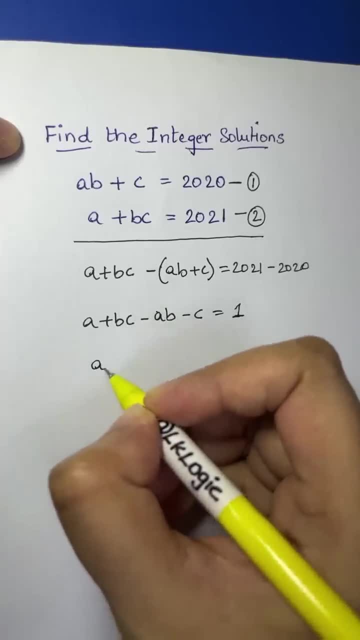 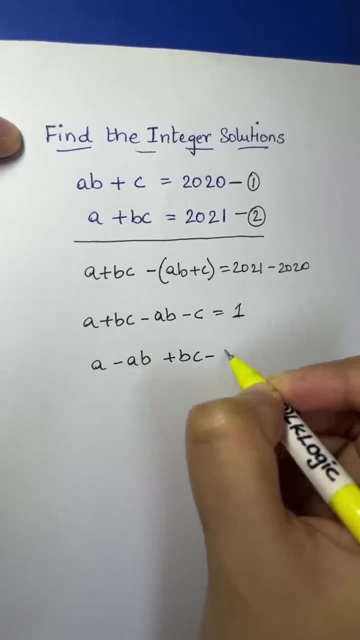 this. So let's let's bring the terms one side: a minus a, b. I can see a common in this. that's why, plus b, c, minus a, I can see a- c common in this. So let me split up the terms. Yes, now I can take. 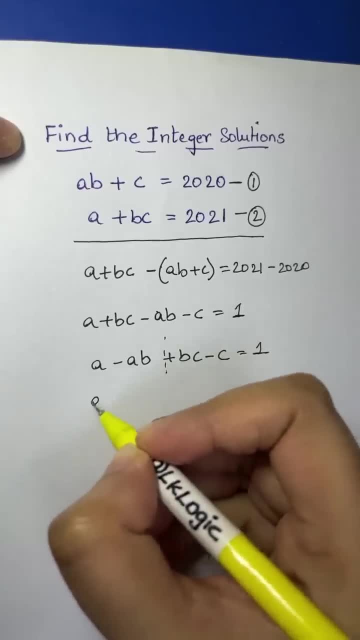 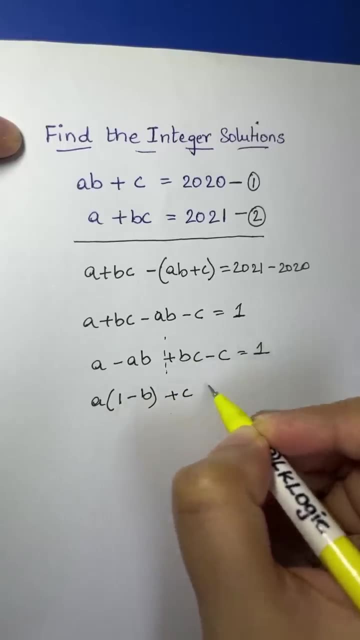 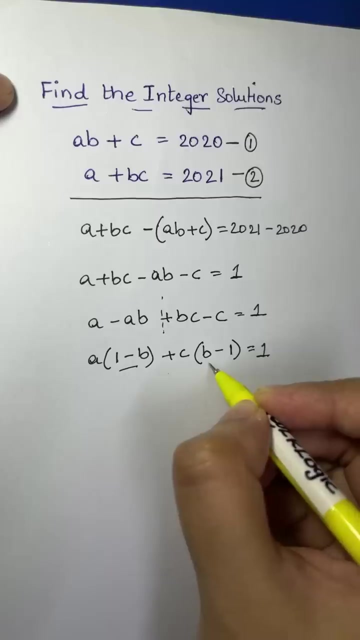 out the greatest common factor between them. So here I can find it: a is common, So left is one minus b. And here I can see c is common, plus c into b is left. b minus one equals to one. All right now, what do we have? Here we have one minus b, and here we have b minus one. 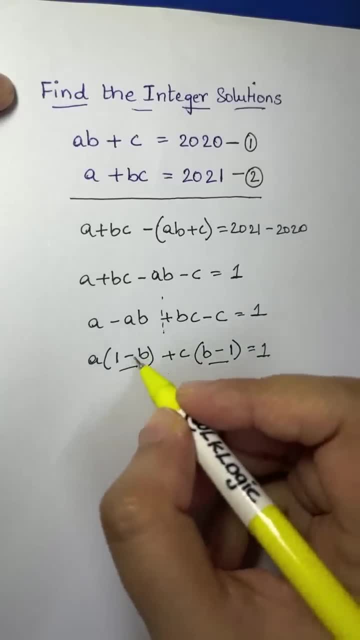 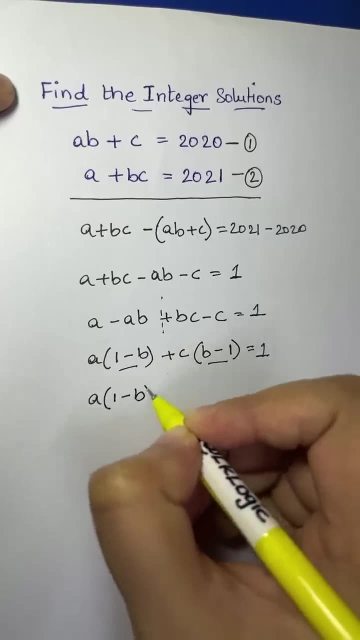 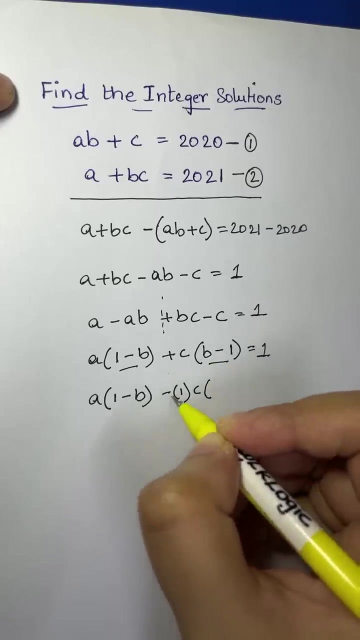 I cannot take it out common because there's a difference of signs. So what do I do? is I take out the minus sign common. So here I have a one minus b. Take out minus one common and c that will be minus into minus. should give you. 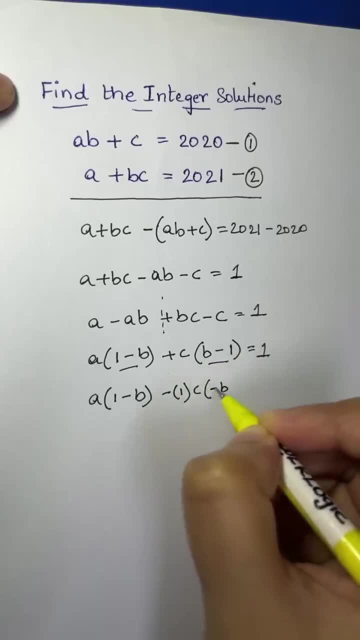 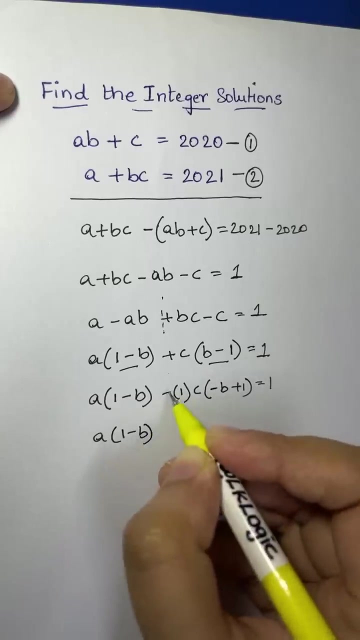 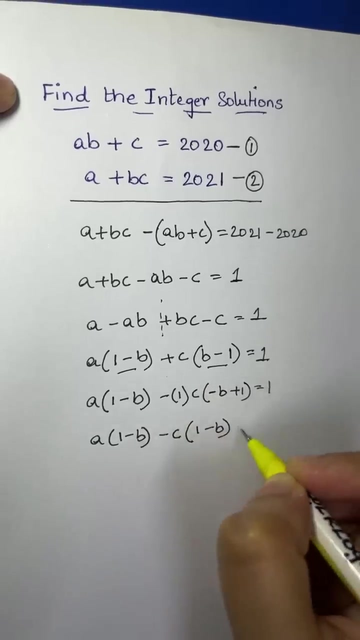 plus b. So we'll have a minus b. minus into minus should give you plus b, And then minus into plus one should give you minus one equals to one. So what did it become? One minus b. I can write it: one into c is minus c times one minus b. So I made it same like this: one equals to one. Now I can. 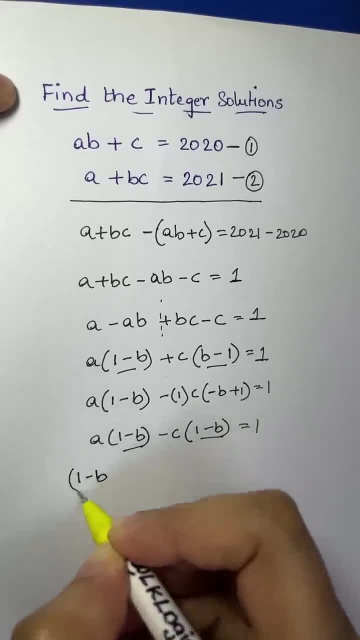 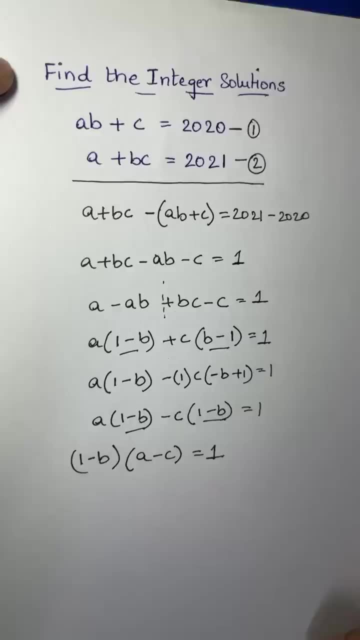 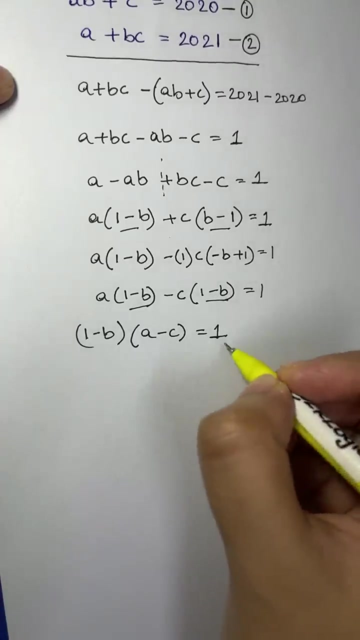 take out one minus b common in this. So one minus b into a minus c equals to one. All right, so now we have solved this part. We have to find out the values of a, b and c. Basically, your answer is one, but it has two solutions. 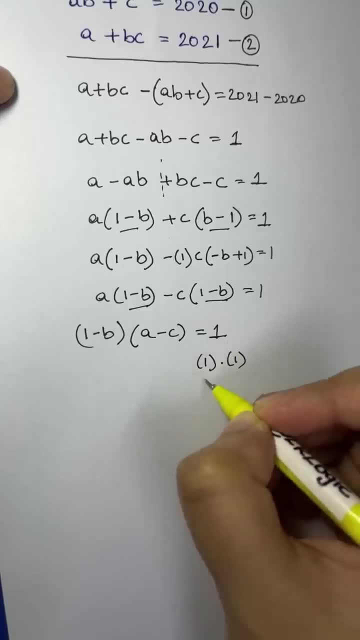 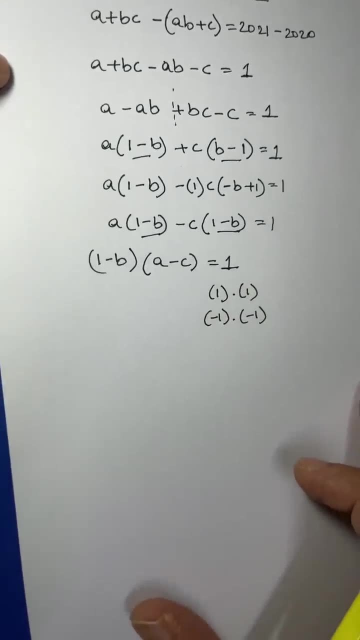 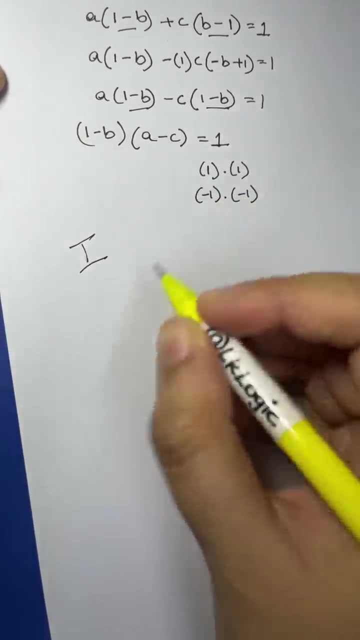 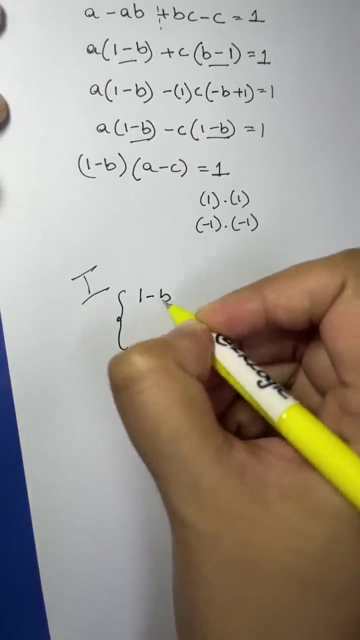 So you have one minus b equals to one into one. You can write it as this: And negative one times negative one also gives you positive one. Now what do we do? So we have two solutions. Now let me write that down. The first one is you have one minus b, So you have one minus b equals to one. 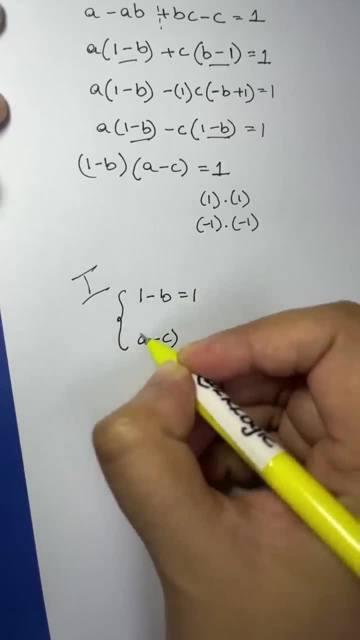 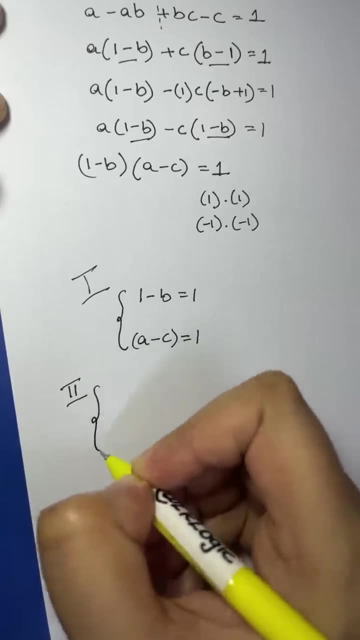 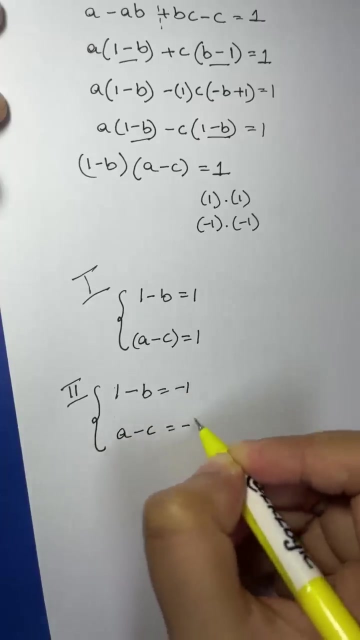 And then you have a minus c. Okay, And the second one You have: one minus b equals to negative one And a minus c equals to negative one. So let's solve what will be the answers for this one. One minus b equals to one. 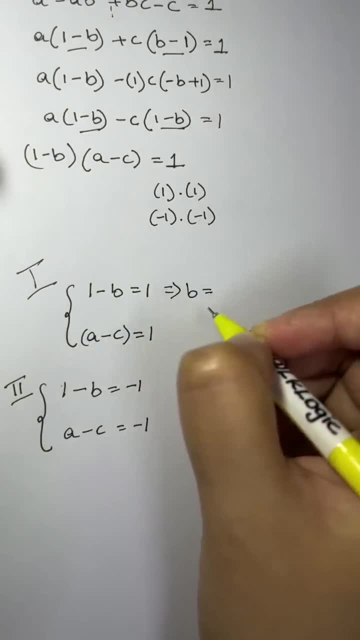 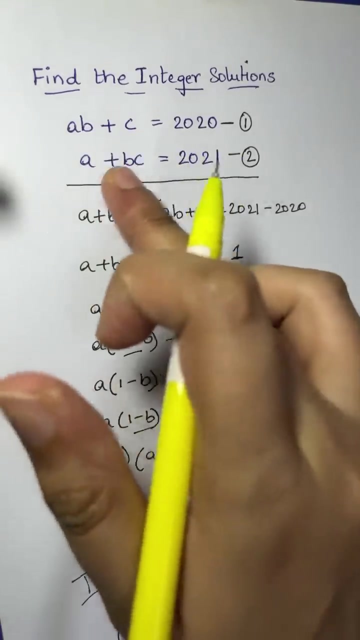 So what will be the value of b? here? b is equal to b is equal to zero. One minus one is zero, So your b is zero. Then what will be the values of a and c? So when you have this, you are going to just substitute into a plus b. What were the equations? we have? a b plus c equals to 2020.. 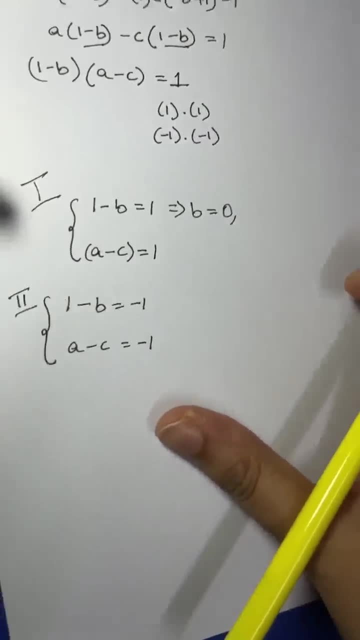 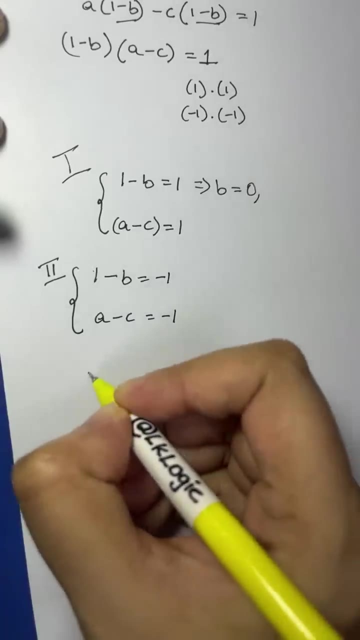 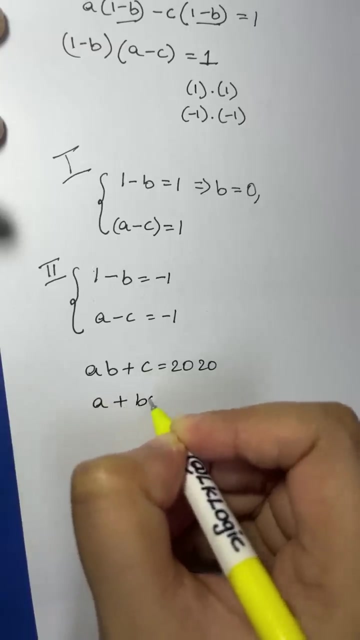 a plus b c equals to 2021.. So let me just write down here: We have a b plus c, We have a b plus c, and a plus b c equals to 2021.. Now let's substitute: b equals to zero in both the equations. 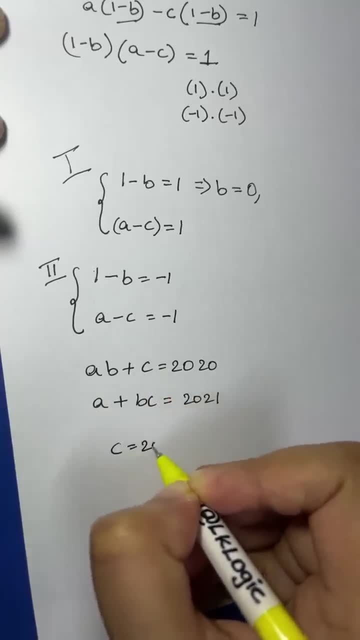 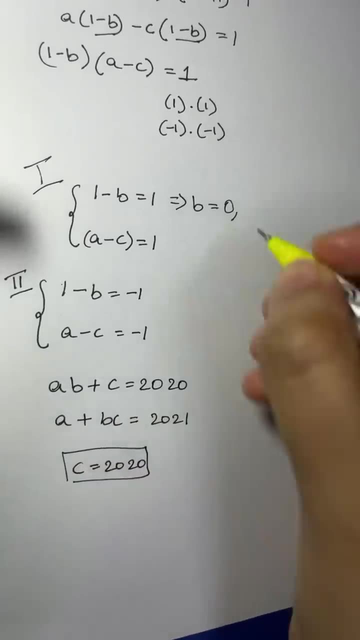 For in first one we are going to get c is equal to 2020.. When you substitute b equals to zero, you're going to get c equals to 2020.. So that's, that's right: c is equal to 2020.. Now let's. 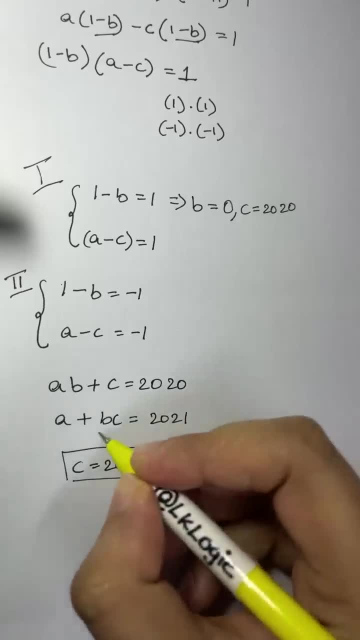 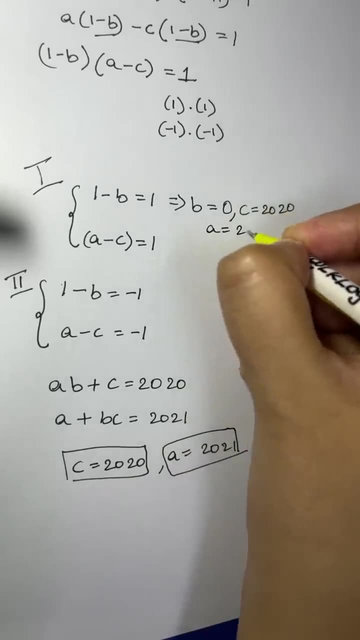 substitute in the second equation, b is equal to zero. So you have a is equal to zero. So you have a is equal to 2021.. That's how you get. So you get a is equal to 2021.. Okay, now for the second one. 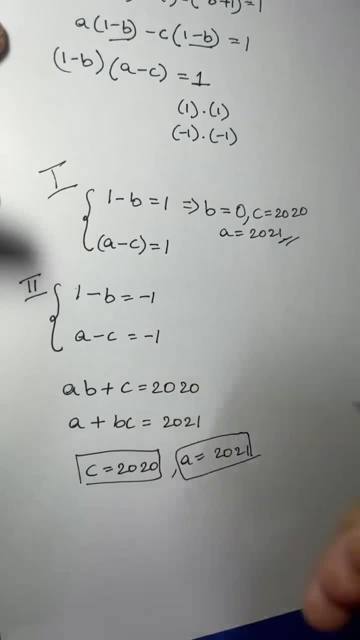 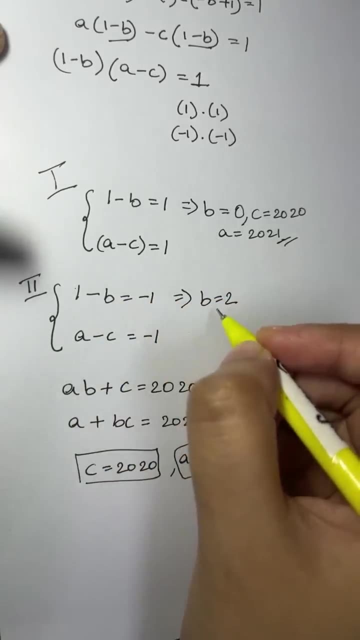 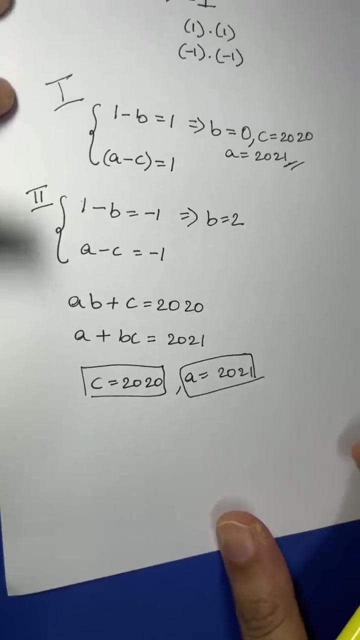 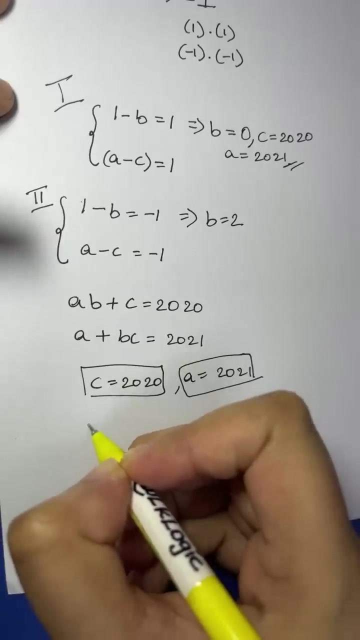 You have, b is equal to two. One plus one gives you two, So b is equal to two. Now how do we find out the values for a? Let's substitute again: b is equal to two in these two equations We are going to have: okay, we are going to have a b plus c. We are going to have two. a plus c is equal to 2020.. 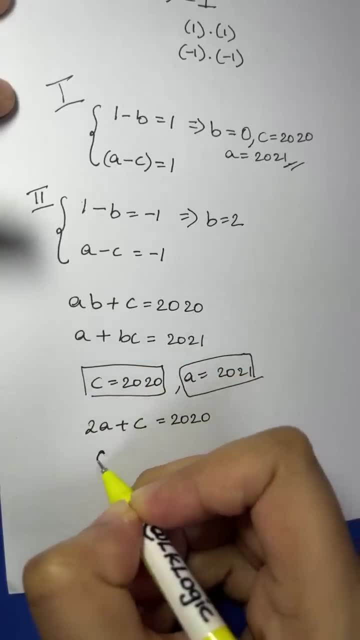 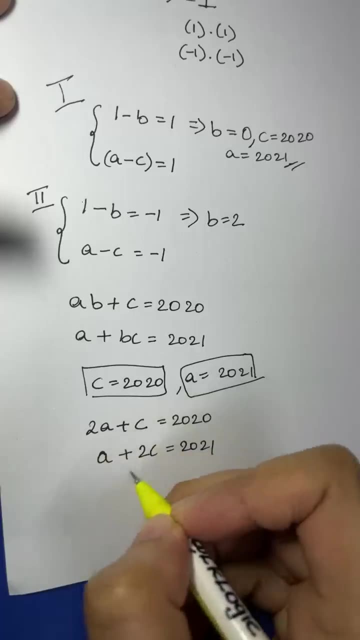 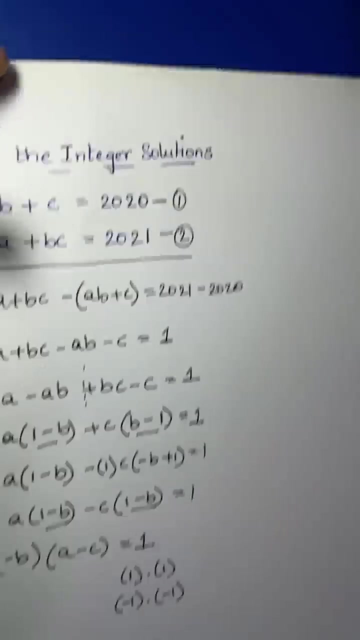 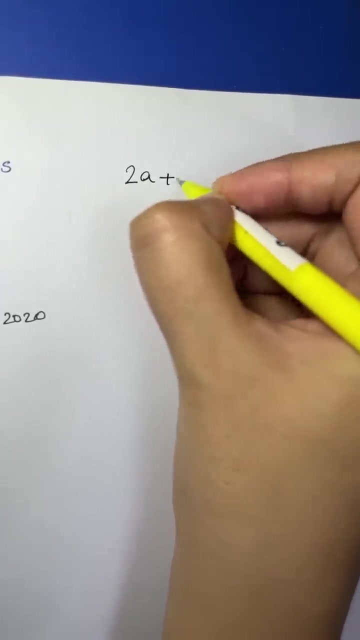 And then you have two. you have a plus two c equals to 2021.. Now these are two equations with two variables, So let us solve either- you can solve it using substitution method or elimination method- Let's solve it, The two equations. I'm going to write that again. That's equal to two. a plus c equals to 2020.. 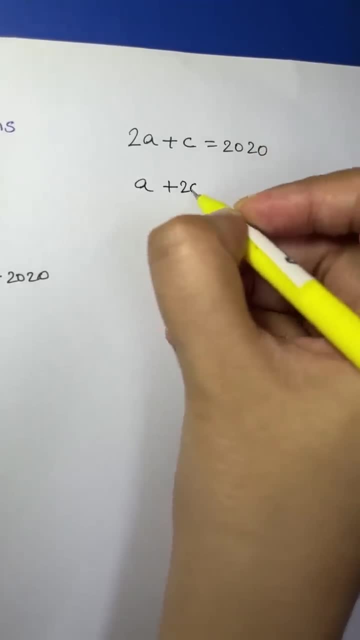 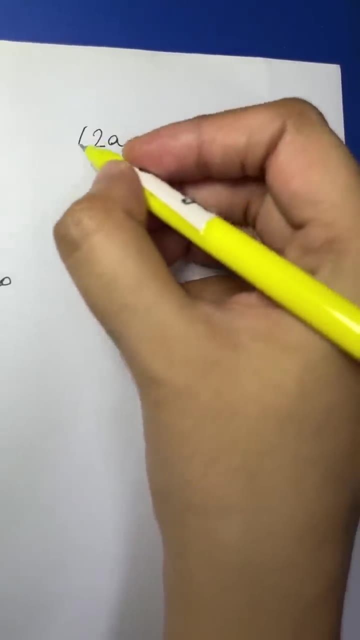 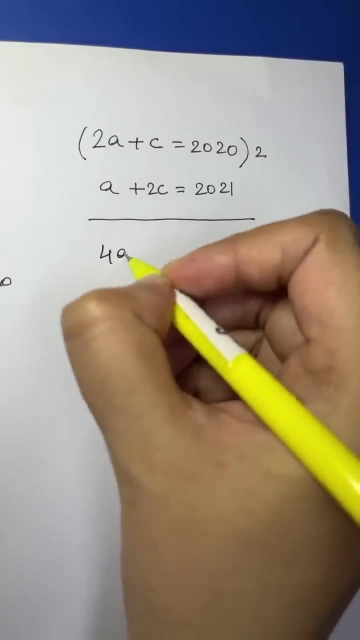 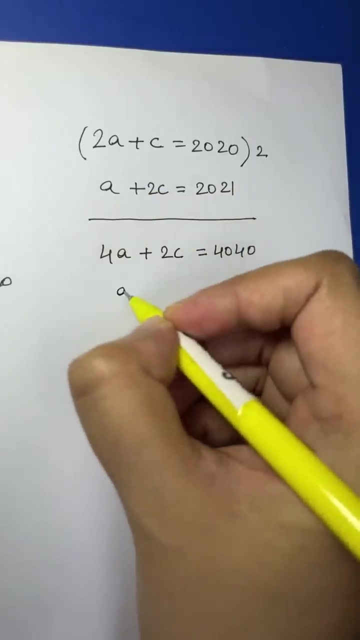 And another equation is: a plus two c equals to 2021.. Now, if you're using elimination method, what you just do: just multiply times two, So you're going to get back four: a plus two c equals to 4040.. Now for this equation, I'm going to write that back: a plus two c equals to 2021.. 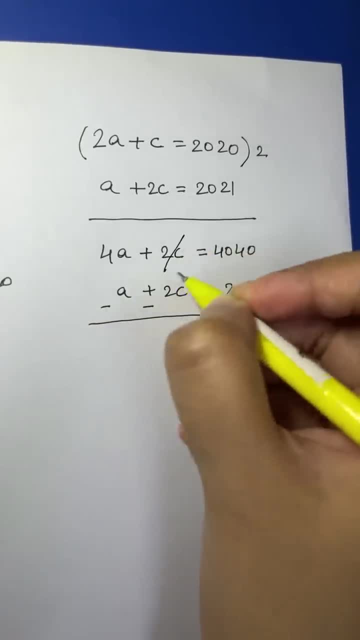 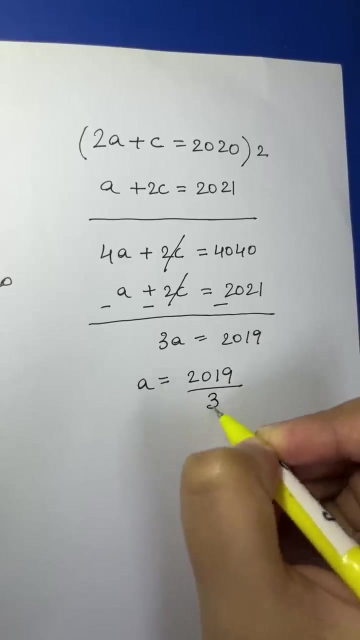 Now just change the sign subtracted. So two c to c gets cancelled out. four a minus a gives you three. a equals to 4040 minus 2021 gives you 2019.. So a is equal to 2019 divided by three. How much is that equal to? 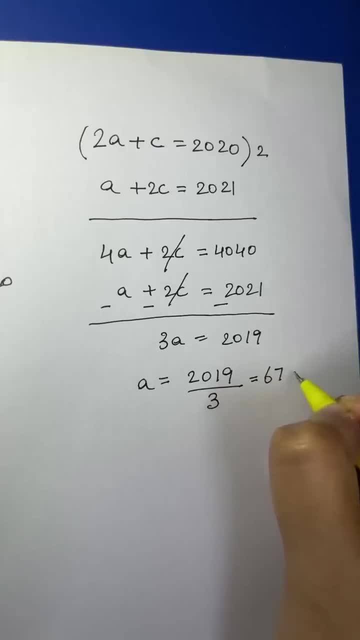 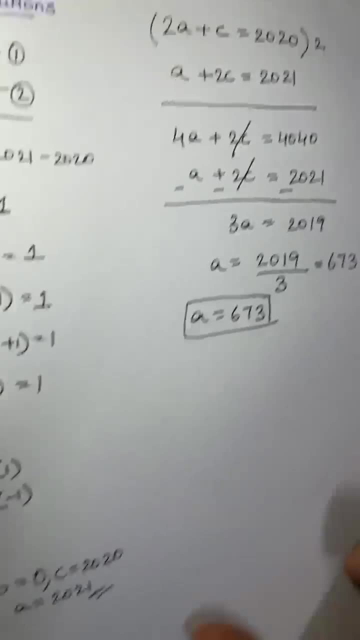 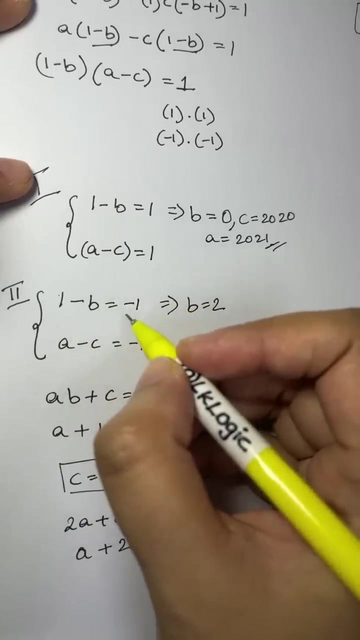 That's 600 n's 673.. So basically, your a is 673.. What will be your b? as we have done this Here, it's given to you One minus b equals to negative one. a minus c equals to negative one. So let's substitute in this a. 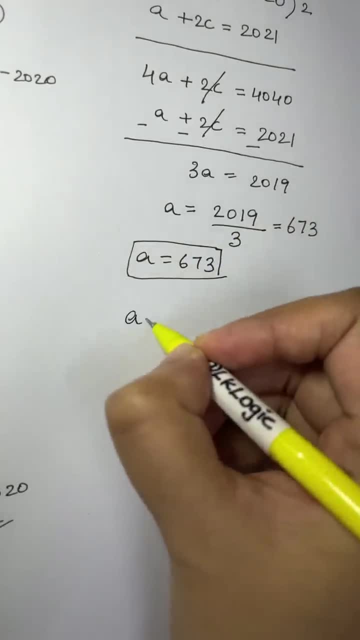 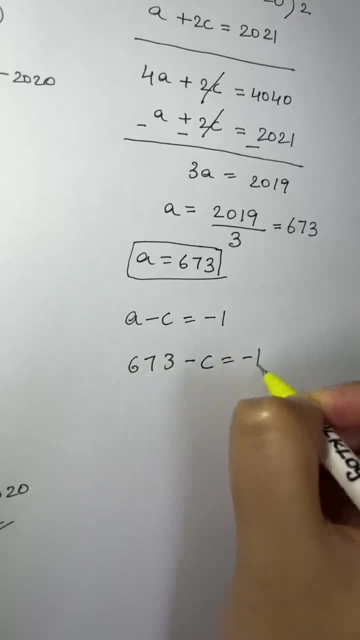 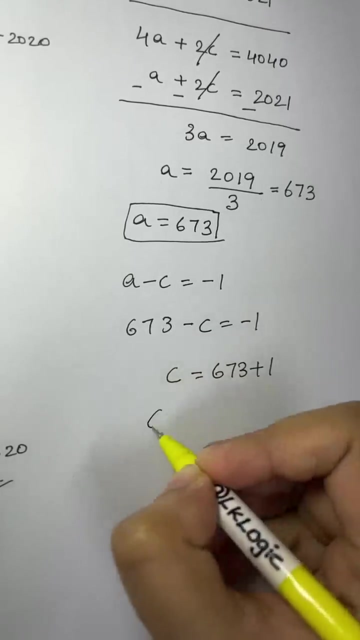 minus c equals to negative one. A minus c equals to negative one. So what is your? a? 673?. Minus b equals to negative one. c equals to negative one. So what is your? c is equal to 673 plus one four. c equals to testimonial study. c equals tostonian.